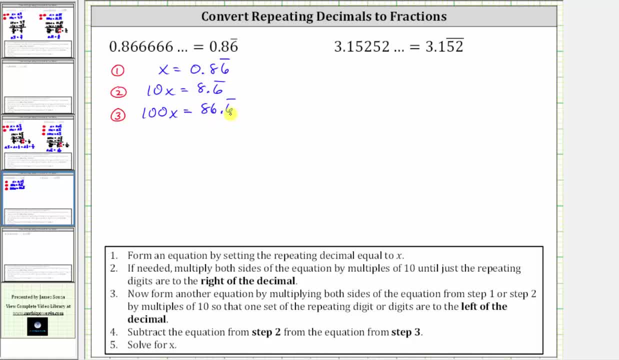 Again. now notice how we have one six to the left of the decimal which is required for step three. Step four: we now subtract the equation from step two from the equation from step three. So, beginning with equation three, we have 100x equals 86.6. repeating: 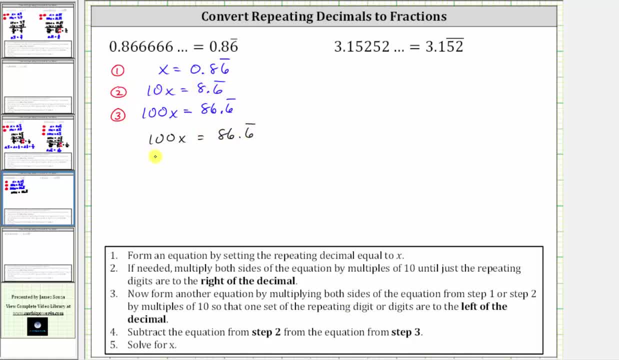 and now we subtract equation two, which means we subtract 10x from the left and we subtract 8.6 repeating on the right. And now we subtract 100x minus 10x is 90x On the right: 86.6 repeating minus 8.6 repeating. 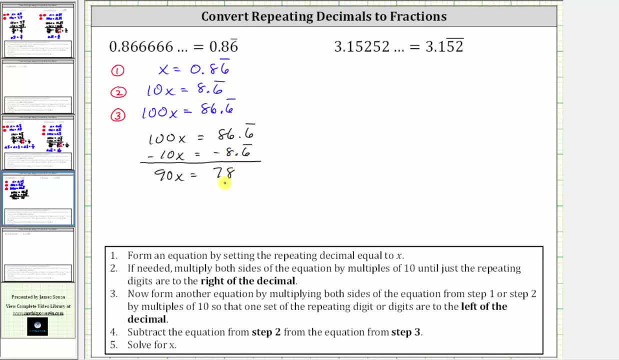 is equal to 78.. And now we solve for x by dividing both sides by 90.. Simplifying on the left, this quotient is one. One times x is x. We have: x equals 78, 90ths, which does simplify. 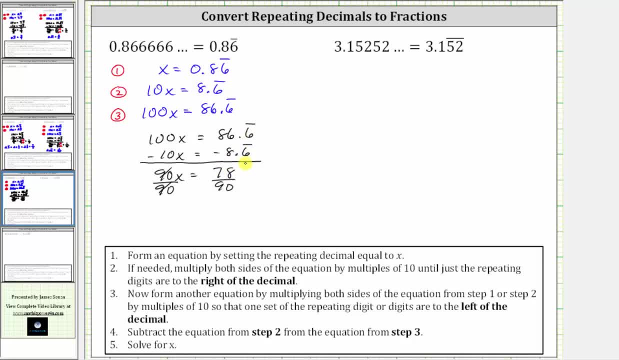 78 and 90 share a common factor of two. So we divide the numerator and denominator by two. 78 divided by two is equal to 39.. 90 divided by two is equal to 45. Now we have: x equals 39, 45ths. 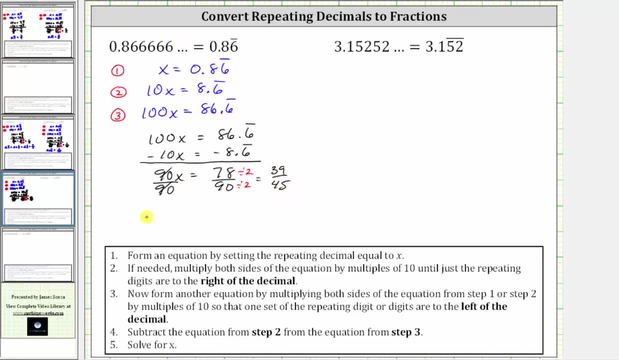 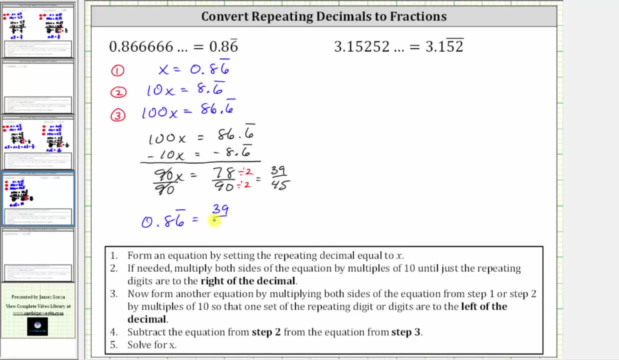 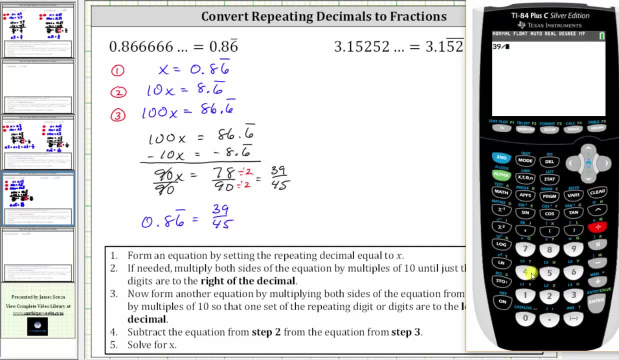 With the six repeating is equal to 39, 45ths, And of course we can easily check this on the calculator. 39 divided by 45 does give us the repeating decimal of 0.86. with the six repeating Next, we have 3.152 with just the five and two repeating. 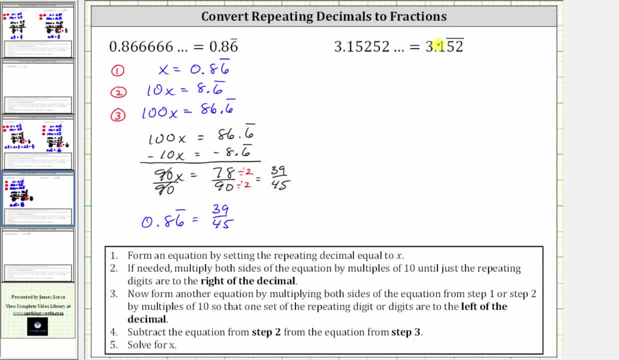 Step one, we set x equal to the repeating decimal, So we'll leave off the three for right now- and the equation is: x equals 0.152, with the five and two repeating. This is equation one. For equation two, we multiply both sides of the equation. 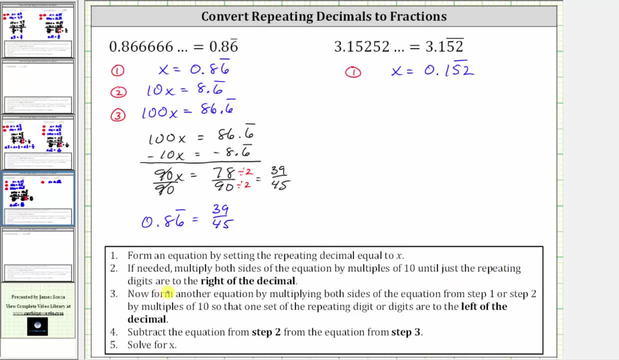 by multiples of 10 until just the repeating digits are to the right of the decimal. Notice, right now we have this one to the right which doesn't repeat. We only want the five and the two to the right, which means we'd have to move the decimal one place. 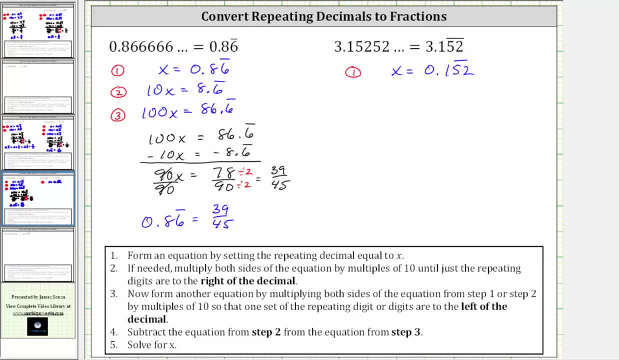 to the right, which is equivalent to multiplying by 10.. multiplying by 10.. So for step 2, we multiply both sides of the equation by 10.. 10 times x is 10x and 10 times 0.152, with the 5 and 2 repeating is: 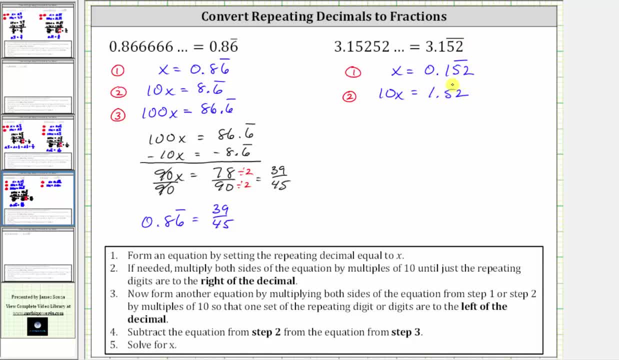 equal to 1.52, with the 5 and 2 repeating. Notice how just the repeating digits are now to the right of the decimal Step 3,. we now form another equation by multiplying both sides of the equation- from step 1 or 2, by multiples of 10. so 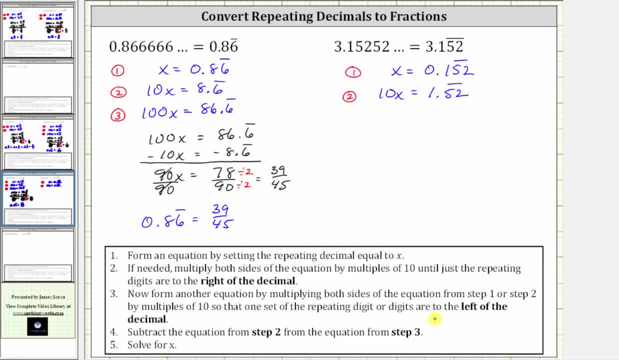 that one set of the repeating digit or digits are now to the left of the decimal, Which means now we want a decimal where we have a 5 and 2 to the left of the decimal. In order to do this, we have to move the decimal two places to. 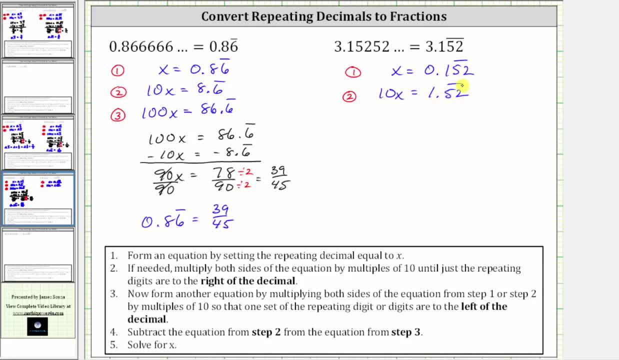 the right, which is equivalent to multiplying by 100.. So for step 3, or equation 3, we multiply both sides of equation 2 by 100, we flipping and multiplying by 10 to the right phenomena. i had similar news: my 100 times 10x is equal to 1000x and 100 times 1.52 with the 5 and 2. 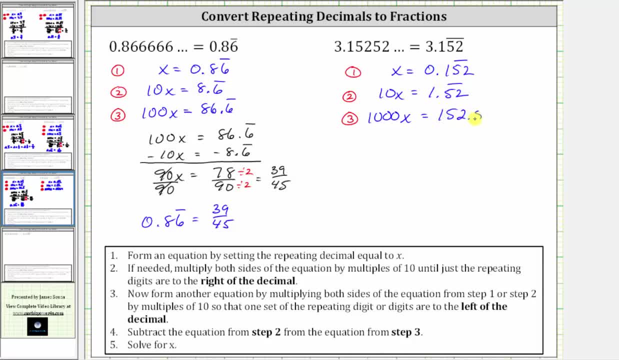 repeating is equal to 152.52 repeating. For step 4, we subtract equation 2 from equation 3.. So, beginning with equation 3, we have 1000x, equals 152.52 repeating, And now we subtract equation 2.. So we subtract 10x. 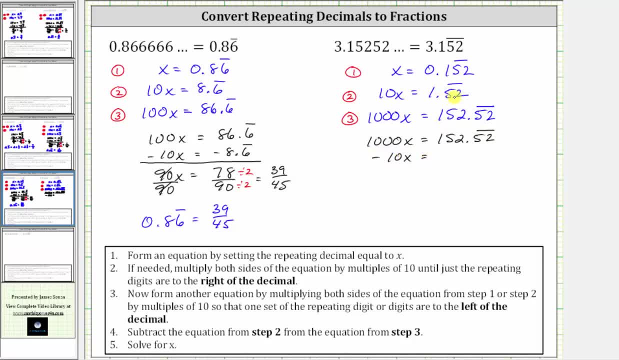 on the left and we subtract 1.52 with the 5 and 2 repeating on the right. Subtracting 1000x minus 10x is 990x equals, subtracting on the right, 152.52. repeating minus 1.52. repeating is equal to 151.. And now we